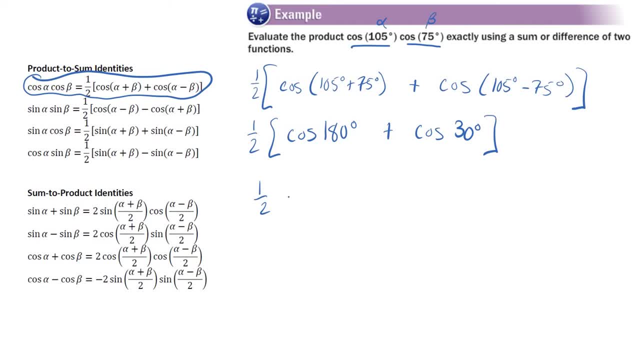 Hey, 180 and 30 are both on my unit circle, So let's see what happens here. So, cosine of 180, if you look at your unit circle, cosine of 180 is negative 1.. Cosine of 30 degrees is root 3 over 2.. 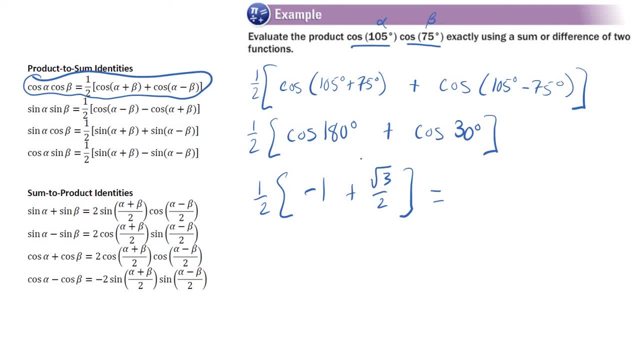 So now let's just simplify this a little bit Again. let's get a common denominator here, And so in fact I guess I could just distribute, But let's combine this first. So this would be negative 2 over 2.. 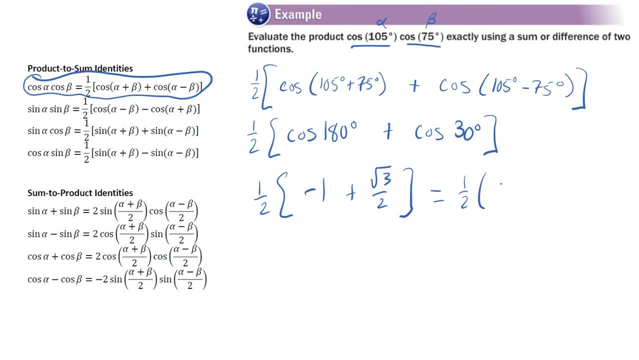 So if I have one half times negative 2 plus root 3, all over 2.. And again, all I did was get a common denominator, Turn that into negative 2 halves, And so now you could distribute, I guess, Or even just leave it like this probably. 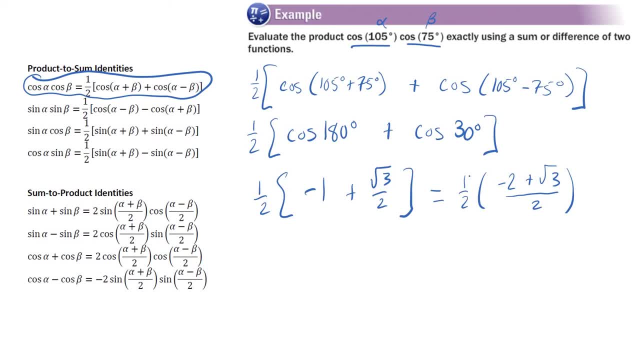 It kind of depends on how they're going to show their answer. In fact, I'll just leave it like this. That's probably fine. The only difference: you put it over 4, right. So there we go. So really not too bad. 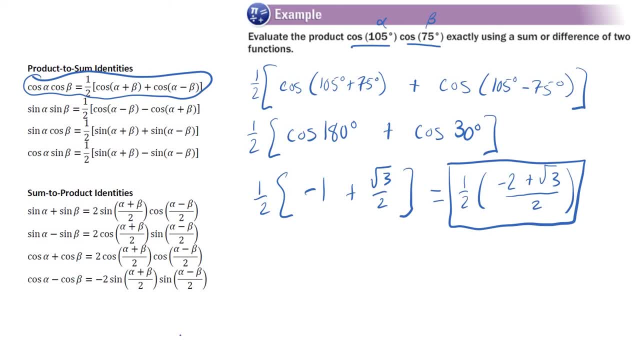 You just apply the formulas. They're basically plug and play, Pretty straightforward. I'm not even going to put any of these on the practice assignment today, But they can be very useful. Want to make sure we're aware of them. Know that we've got another tool out there. 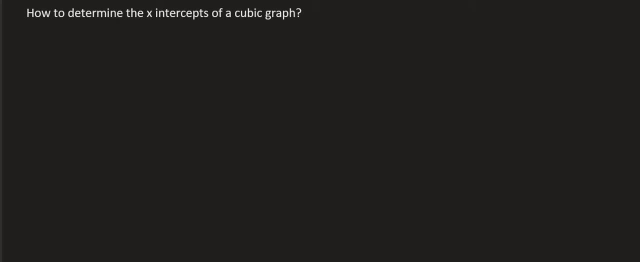 This video is extremely important. In grade 12, we encounter a new type of graph, which is the cubic graph, and that typically looks something like this: To find x-intercepts, we know that you have to make y equal to zero, and then you would typically find three of them for a cubic graph.